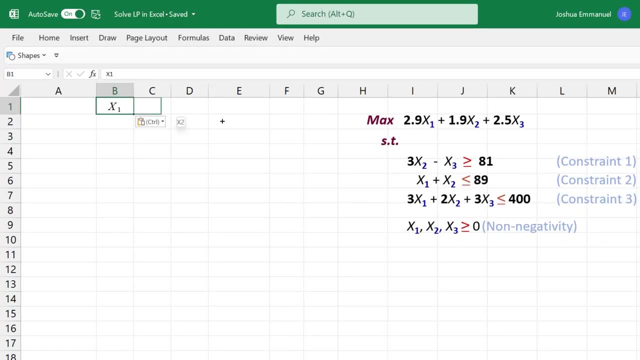 Now I'm going to place X1 here. Drag to the right for X2 and X3.. I'm going to shade the cells beneath them yellow. That's where I want the optimal solution to be placed. Next I'm going to place the objective function. 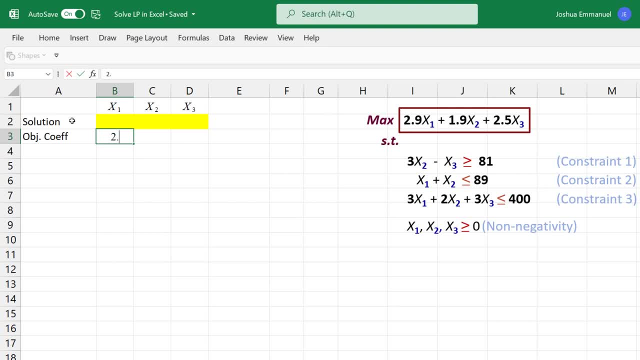 coefficients on this row: 2.9,, 1.9, 2.5.. I'll start the constraints here. Copy down for 2 and 3.. For constraint 1, the coefficient of X1 is 0, so we can either enter 0 here. 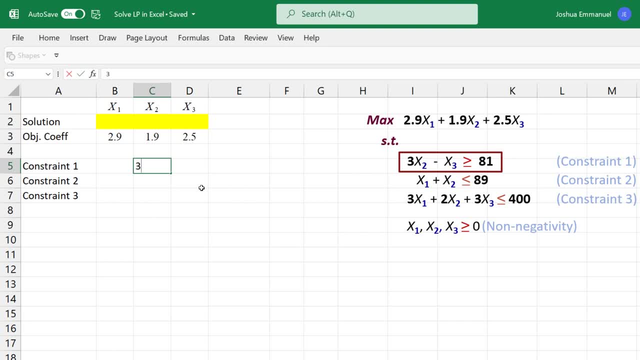 or just leave it blank. The coefficient of X2 is 3, and for X3, it's negative. 1.. For constraint 2, the coefficient of X1 is 0, so we can either enter 0 here or just leave it blank. 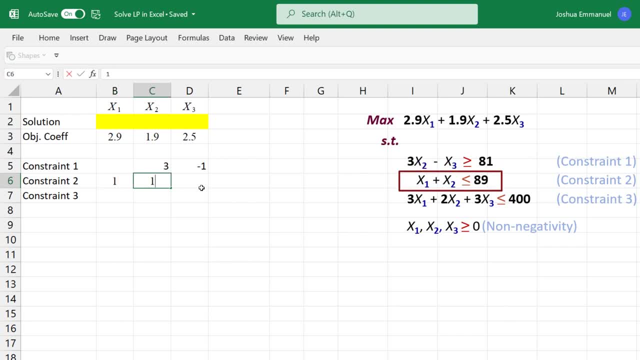 The coefficients are 1 for X1, and 1 for X2.. For constraint 3, we have 3,, 2, and 3.. Next we set up a formula for the objective function Z. Recall that these yellow cells are set up to hold the values of X1,, X2, and X3. Thus, 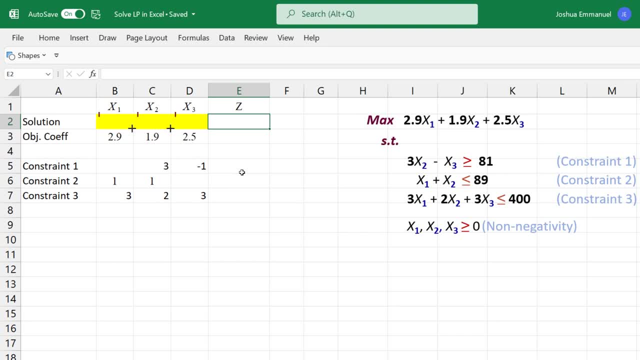 the objective function will be the sum of the product of each coefficient and the yellow cell above it. Now let's go back to our model to see where we can put the value of the new coefficient. Let's take our circle on the left here. 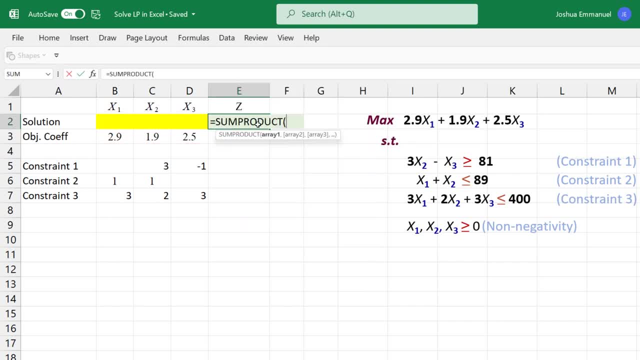 2.9, 1.9,, 1.9, 2.5.. I'm going to color the cell light green and use equals. SUMPRODUCT. Select the coefficient comma, then select the variable cells. Enter The value is zero here because we are currently multiplying the coefficients by zero in the 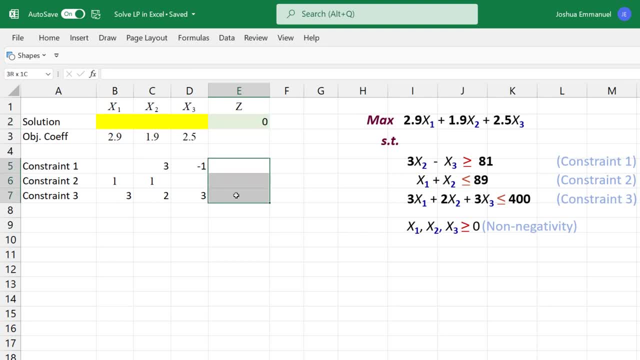 variable cells. I'm going to color the constraint formula cells blue. here and again, use equals SUMPRODUCT, Select the coefficient comma, then select the variable cells. This time I'm going to lock the variables down using the F4 key on Windows. 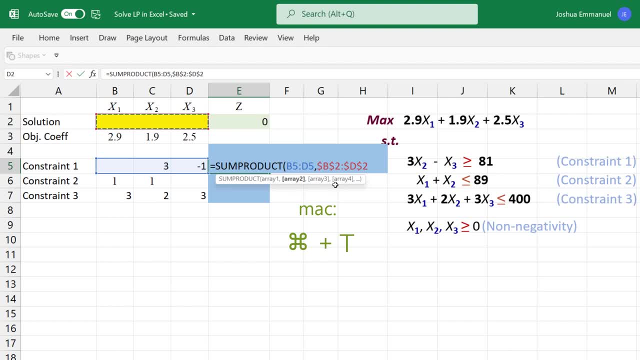 On Mac, use command T. You can also manually type the dollar signs. Use the fill handle to copy it down And double click it on. the last one here shows that the formula copied correctly. Next I'm going to place inequality signs for each constraint here. 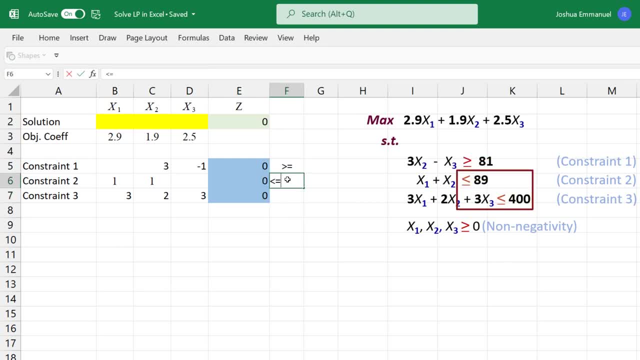 Greater or equal for constraint 1, and less or equal for constraints 2 and 3.. The formulas in blue here represent the constraints left and side. For the right hand side we have 81 for constraint 1,, 89 for constraint 2, and 400 for constraint. 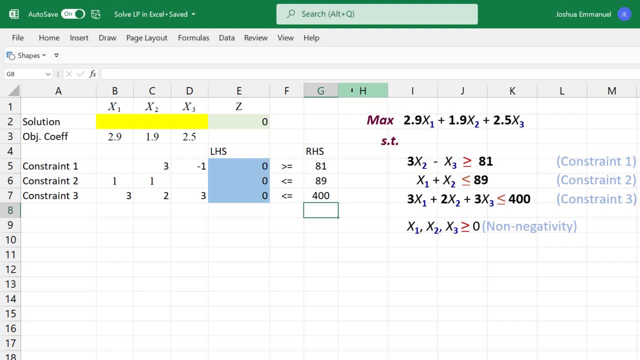 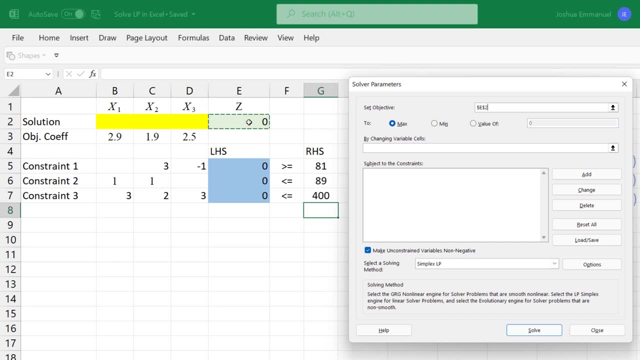 3. The setup is now complete. Now to solve this, I'm going to click on the Data tab, then click Solver. For the objective I'm going to select the objective function formula For changing variable cells. select the yellow cells. 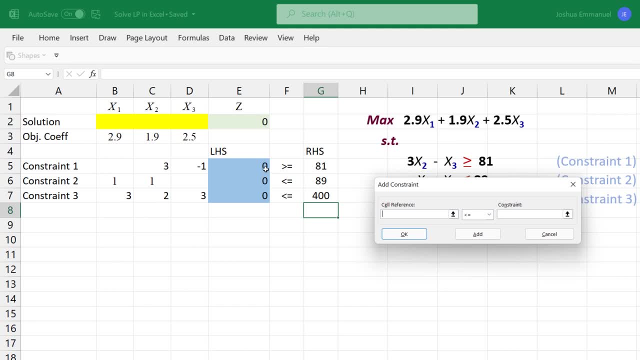 To add the constraints: click Add For constraint 1,. click the left hand side for cell reference. Change the sign to greater or equal and select the right hand side for the constraint value. Click Add For constraint 2, select the left hand side. 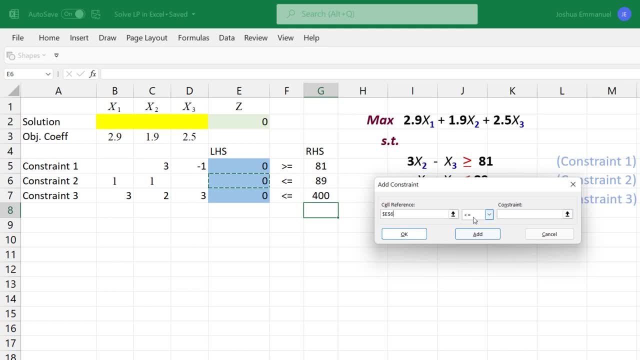 The sign is already less than. In fact, both constraints 2 and 3 are less than constraints, so we can select both left sides at the same time And also select both right sides at the same time. Since that's all the constraints we have, I can click OK. 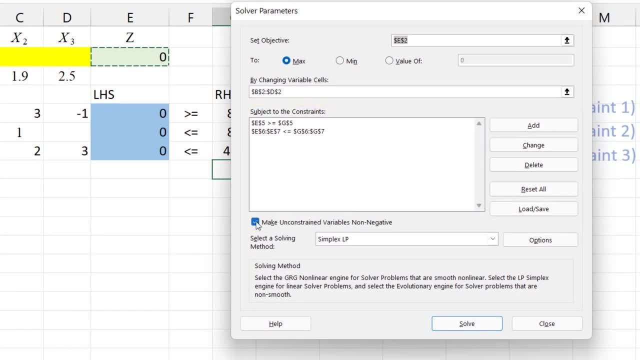 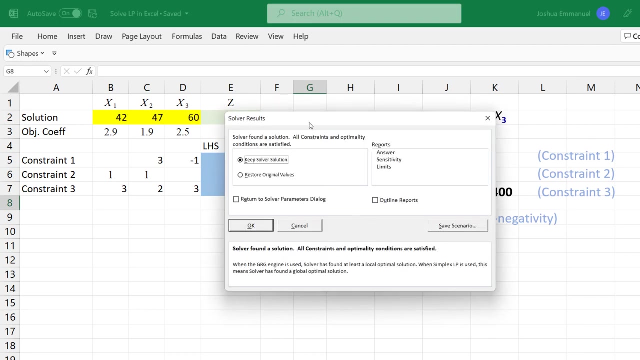 The added constraints appear here. Next, ensure that this non-negativity box is checked And that the solving method is SimplexLP, Click, Solve. The colored cells are now populated with values, With the optimal solution here and the objective function value here. 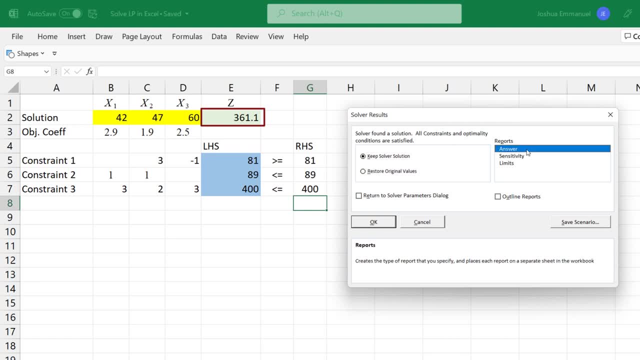 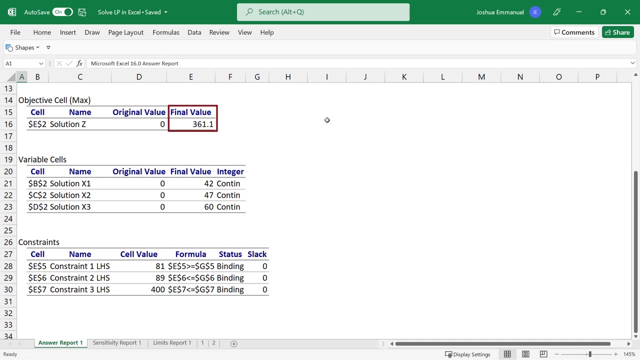 You can stop there and click OK in this dialog box if you're only interested in the optimal solution. Otherwise you can select whichever of these reports you want to see. I'm going to select all three And click OK. The answer report shows the optimal objective function value here. 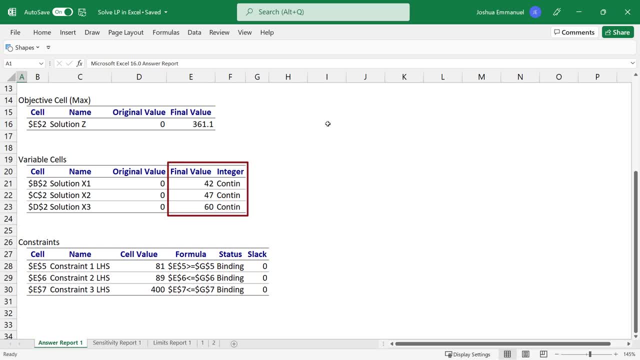 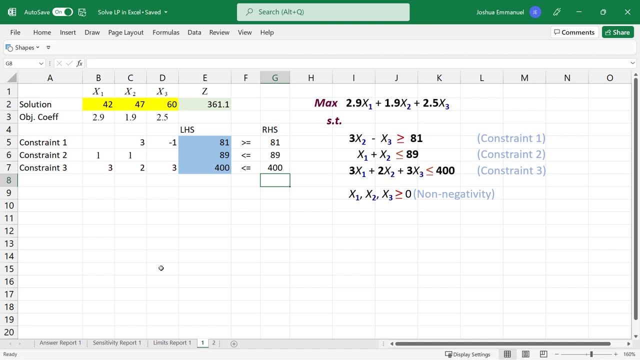 The values of the decision variables at optimal solution here, And if a constraint is non-binding, you will see a positive value for its slack or surplus here. You can also view the sensitivity report and limit reports here, if needed. And that's it for this video. 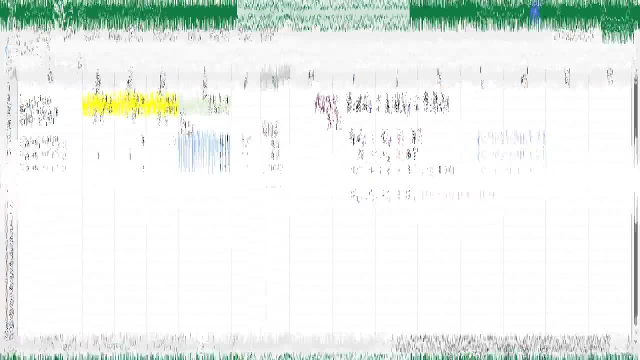 Thanks for watching. I'll see you in the next video.